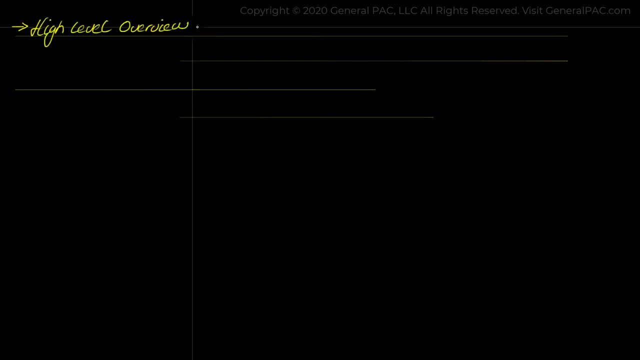 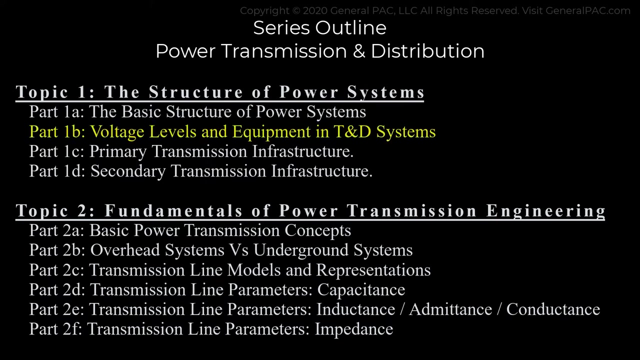 And in this part we will give you a very high-level overview of the basic infrastructure on which the electrical power system is built. In Part 1A, of course, We talk about the basic structures of power systems And then we move on to Part 1B, where we talk about the voltage levels and equipment and transmission and distribution systems. 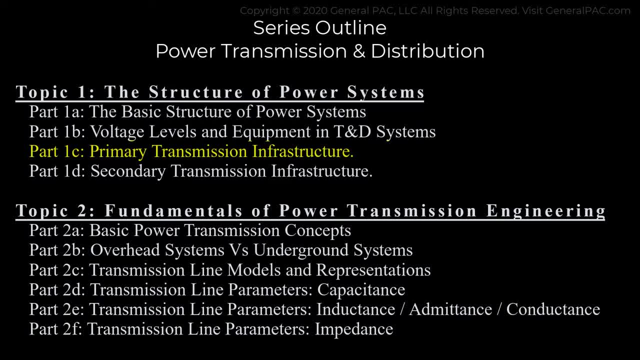 In Part 1C we'll talk about the primary transmission infrastructure And Part 1D the secondary transmission infrastructure, And then there are obviously other related parts, like the fundamentals of power systems, engineering and so forth. Okay, now let's get back to our topic. 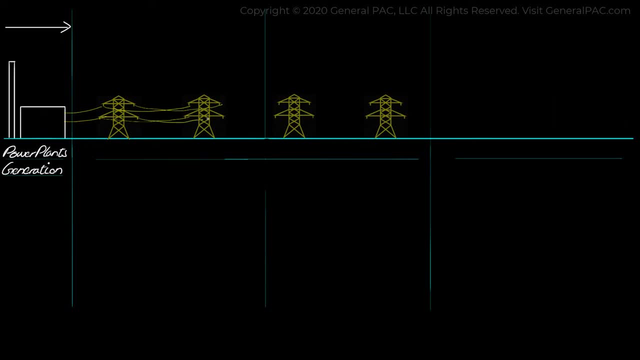 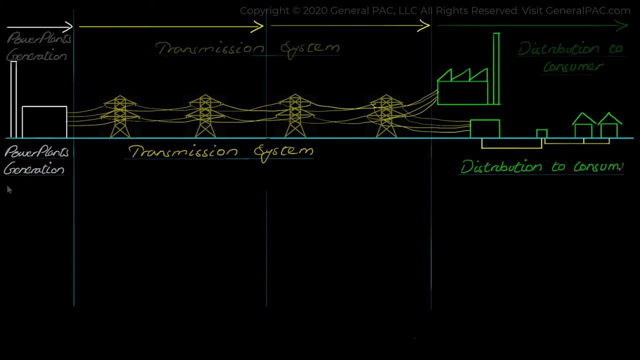 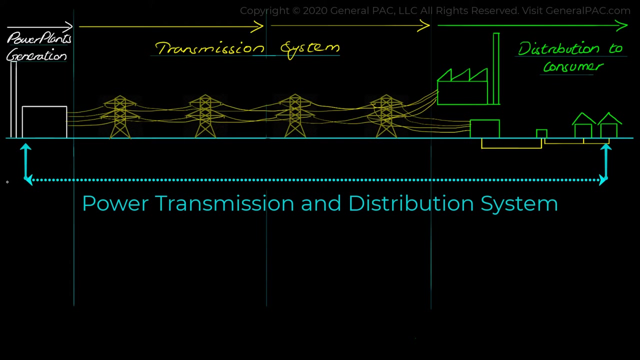 Now traditional power plants generate electricity, Then this electricity is transferred through the transmission system and then distributed to different consumers that use electricity for different purposes. Now, collectively, the whole system involved in power delivery is known as the transmission and distribution system. So the structure of power system comprises of numerous components, like the generating stations. 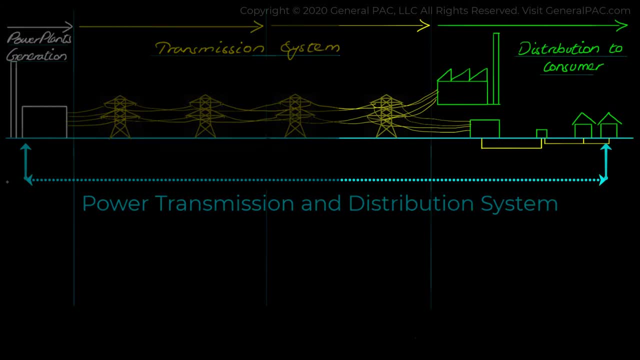 high voltage power transmission lines, different types of transformers, substations, distribution networks and feeder schemes, and then there are also the power systems that are used to generate electricity, And there are alsokh istovisance, and there are also protection devices. 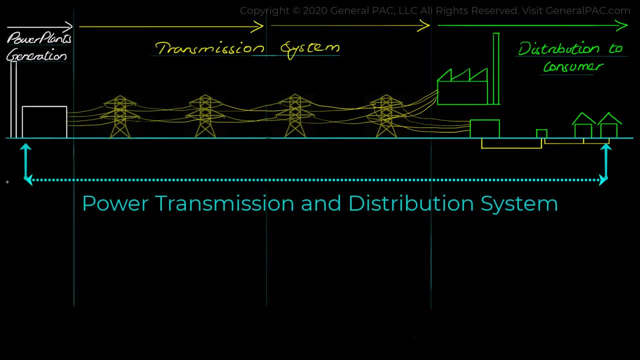 and so forth, And we are focusing on the subject related to T and D, or transmission distribution systems. specifically in this series. Let's draw a representation of a traditional power system. Immediately after traditional power generation, we have the transmission system, We have the power generation system. 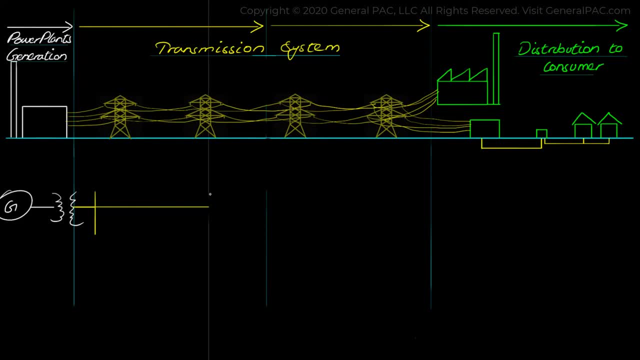 The transmission system is a three-phase network And we use this term network when we have more than one path between any two points. And we use this term network when we have more than one path between any two points, Since it connects calib prior and posterior. this will generate electricity. 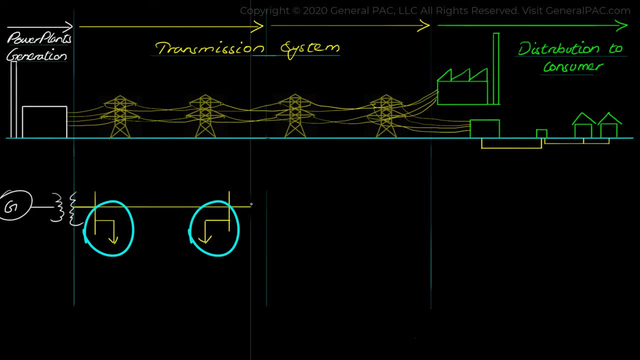 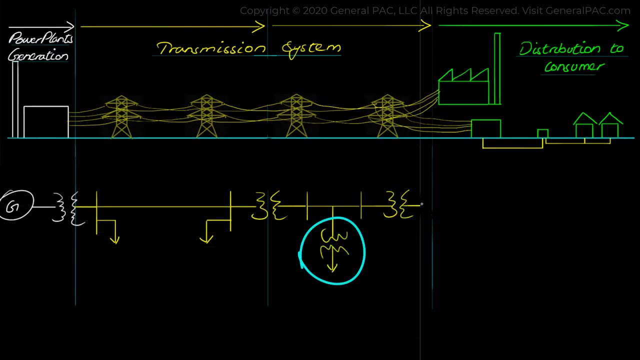 a power source and load through multiple routes, And the main function for which transmission system is responsible for is to deliver bulk energy from the generation side to the consumer end And, furthermore, it provides multiple links for interchange of energy among different interconnection points. 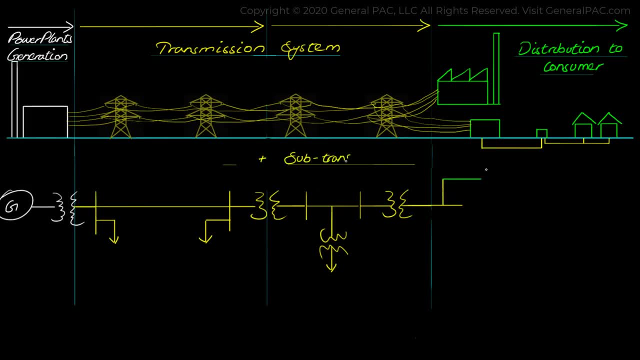 Then there comes the sub-transmission system. It steps down the voltage to a lower voltage level and some of the power through here is directly supplied to heavy industries and few large consumers, while the remaining power is delivered to a distribution system. The sub-transmission system is followed by the distribution system.